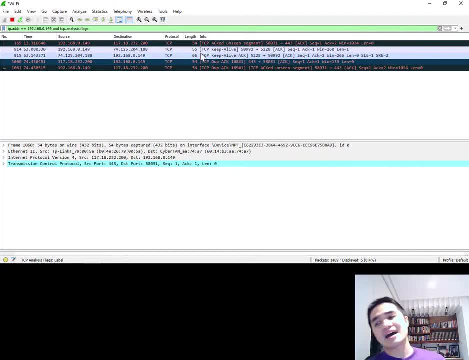 issues. So see, when you see these duplicate acts, these are things where we're having drop packets or we're having some issues on TCP. So this will allow us to see device traffic that is having issues and then it allows to debug, say there's like a broadcast storm, then we're going to see a lot of ARP traffic. 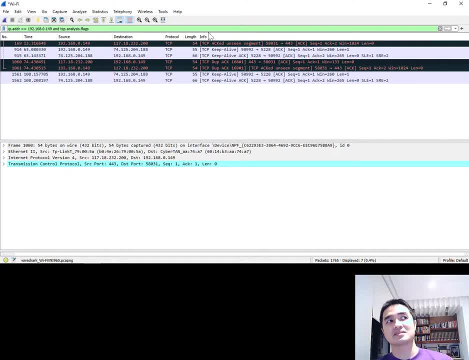 So this is Wireshark- I'm going to press stop and it's pretty hard to see what's going wrong. And the more common one to use, I guess, would be something like the next tool, which would be TeamPlotter. 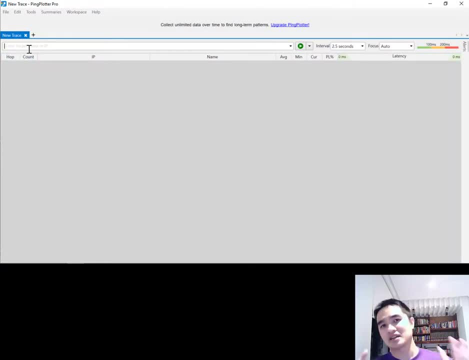 TeamPlotter, TeamPlotter, TeamPlotter just says that because Wireshark has so much data ping, it really gives you the nitty gritty Here. it would just be like the most common problem or drop packets is, just say, one overloaded. 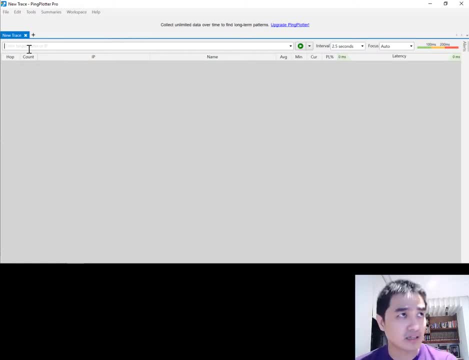 device on the network. So for a tool like that we'd use pingplotterpro or just pingplotter. I'll type a website that I'd want to monitor traffic and then press play, and then what's going to come out is the different hops on the network again. 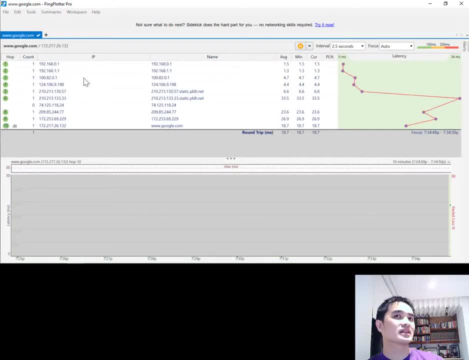 network to get there. So here to get to googlecom, I'm going from the 192.168.0.1 device and then 192.168.1.1,. this is actually my internet router, or the one provided to me by the ISP. 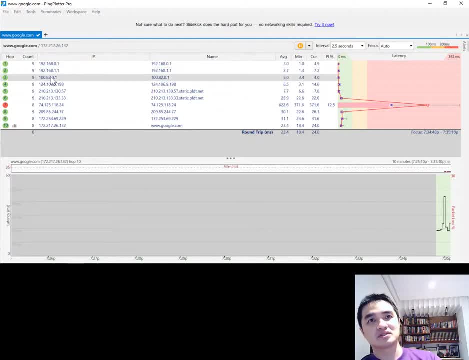 This is the hop from the ISP to the. I guess it's like the switch on my street where we access the IP and then this is all their internal routing. So this is actually a good graph, because we're actually able to see that we're having issues. 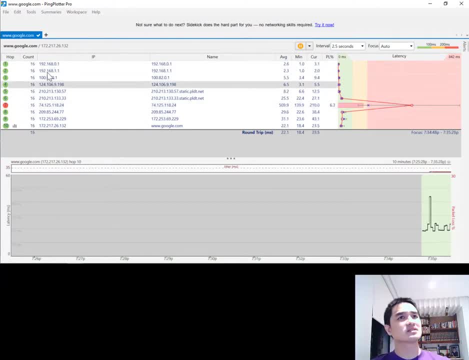 So this is outside of my network, so this is all inside my house: no issues, no packet loss. latency looks good. No packet loss meaning there's nothing happening there, So all the packets are fine. and then suddenly there's 5%. 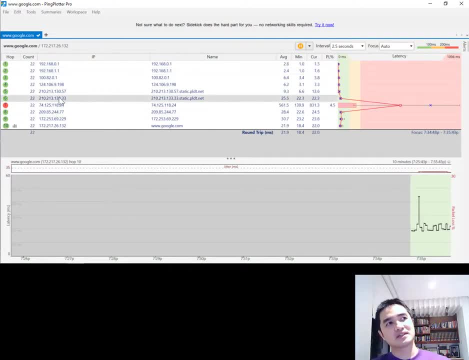 So from this router 210.213.0.1.1,- this is actually my internet router or the one provided to me by Google. So this is the 14.213.0.1.1.3.0.3 to this router 74.125.118.24.. There is a packet loss. 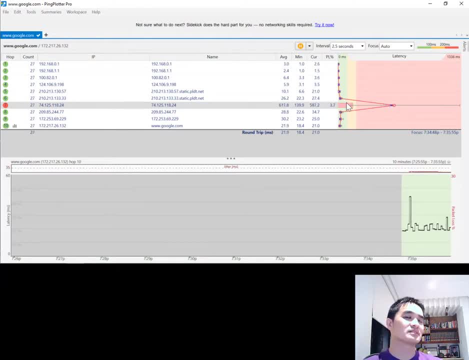 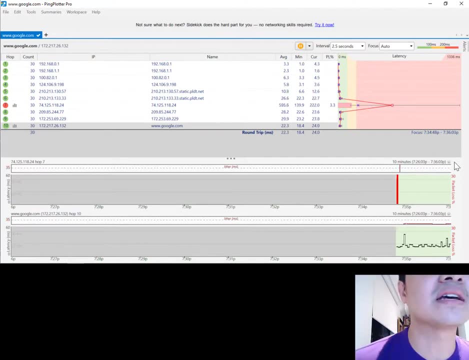 and there is a spike, So we can actually do something like clicking this graph and we can actually see what's happening to that network. So let's just use, say, instead of 10 minutes, let's use something like 60 seconds, and then 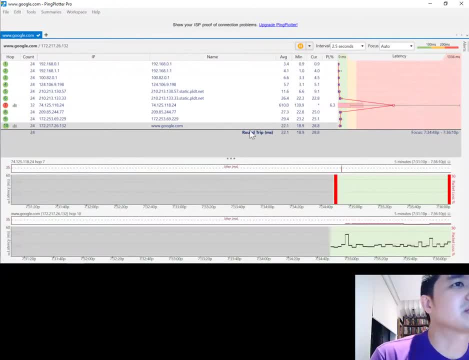 we'll not 60 seconds, do five minutes. Five minutes, and then we'll be able to scroll and see for HOP7, so this is all the way to googlecom. this is what it looks like, but on HOP7 we're. 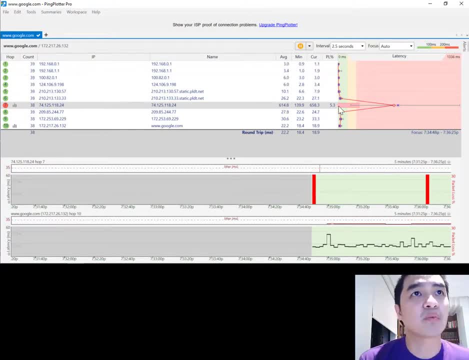 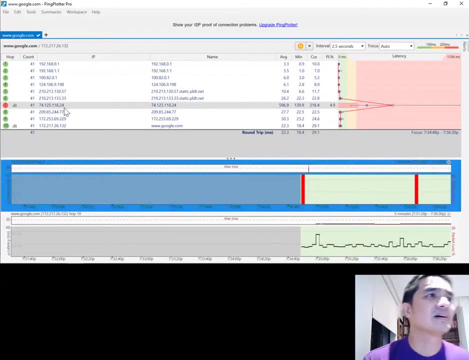 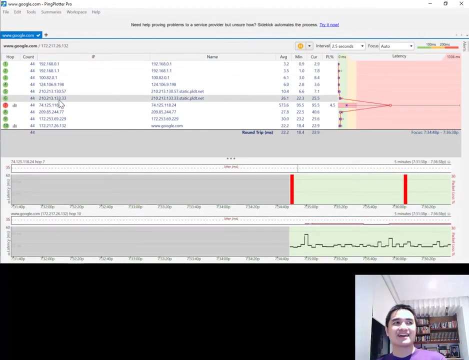 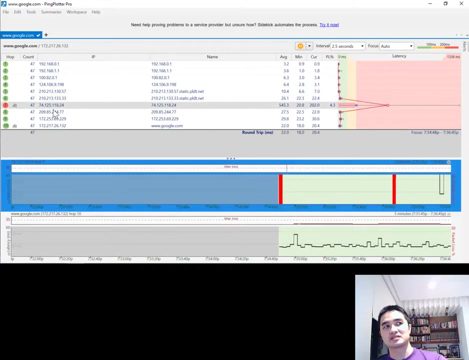 getting a lot of issues, and here we can see that there is a 5.3% packet loss and the latency does come from this link. So I guess, to debug this problem of why is the internet slow, we can actually tell the ISP that it's actually slow because of these two particular routers. 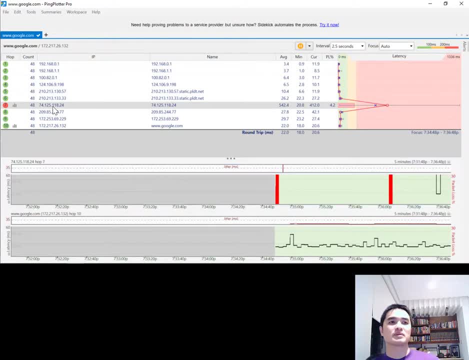 So it's this router that's dropping traffic, probably because it's overloaded, and then at least knowing your network topology, you'd know that when is it your internal network and then when is it your external network. It's good that it also does have a time graph, because I guess the most common reason for 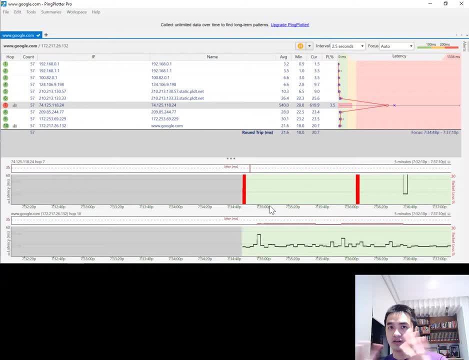 dropped packets would be an overloaded device on the route, Okay, On the network route. So if you leave it for, say, six hours and you come back and you have user complaints, then you can find out. maybe there's a particular process that's happening in your internal. network once an hour and then when that happens, the memory load of a particular HOP or a particular device on your internal route does go haywire or does get overloaded and starts to drop packets. So just call your ISP and here in this issue at least, you can always tell your ISP that. 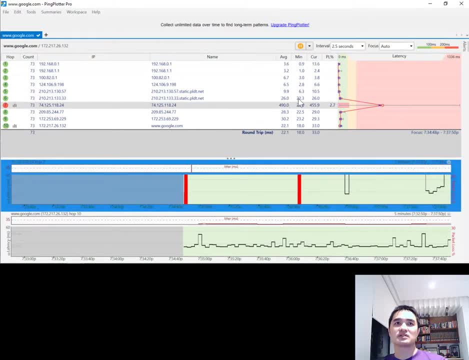 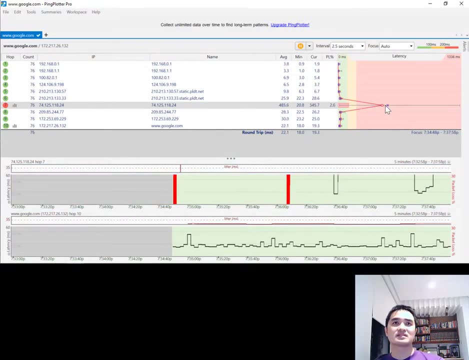 it's these two routers causing the issue, and here you can see consistent drop packets, Okay, So consistent 2.7% and consistent latency issues on this particular HOP. So in this case the issue is not with our internal network, which are these two HOPs. 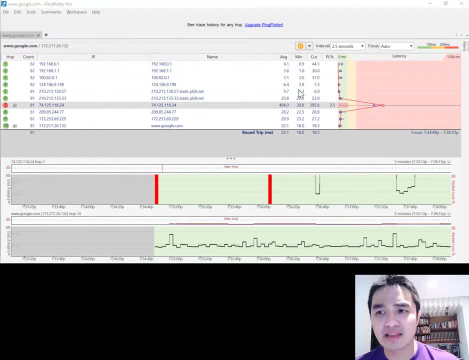 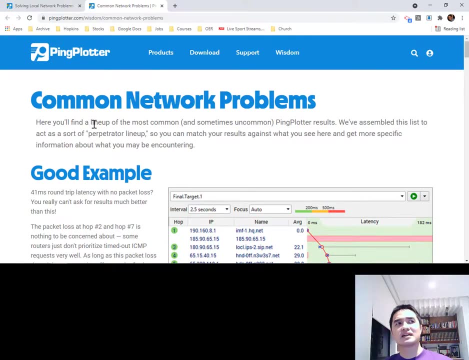 but on HOP number seven, which is the ISP, We're going to go ahead and do a little bit of testing. We're going to go on the last kind of place which would be here. It's pretty good to use plattercom, slash, wisdom, slash, common network problems and they.